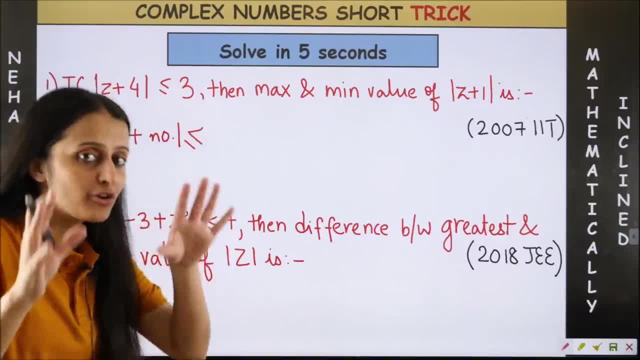 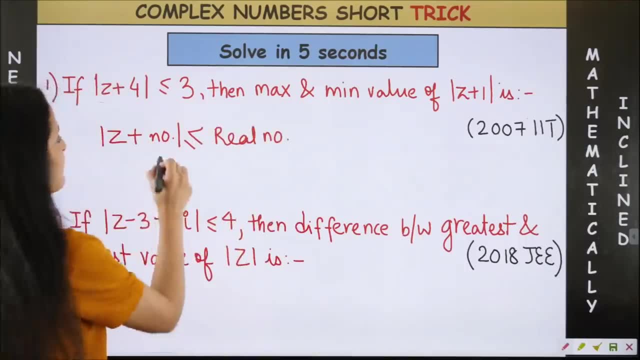 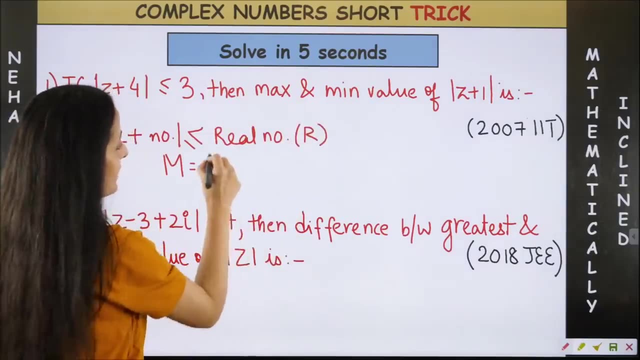 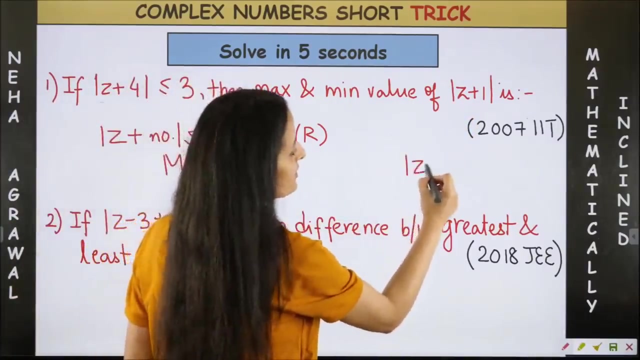 less than equal to. Mind you, not greater than or not equal to, We are strictly going by less than equal to a real number. In that case, your maximum value is this: This r, this real number, which you may call as r okay, plus plus whatever is the modulus you find. That means, like my mod, z plus 1. 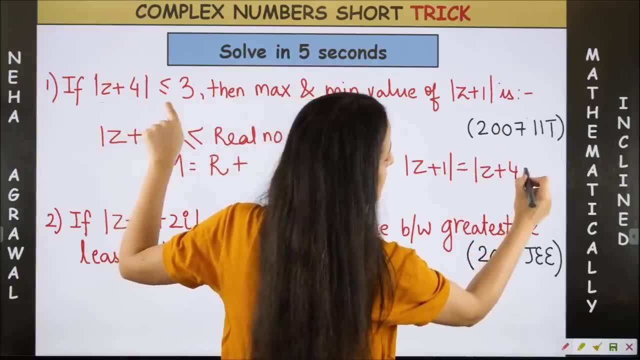 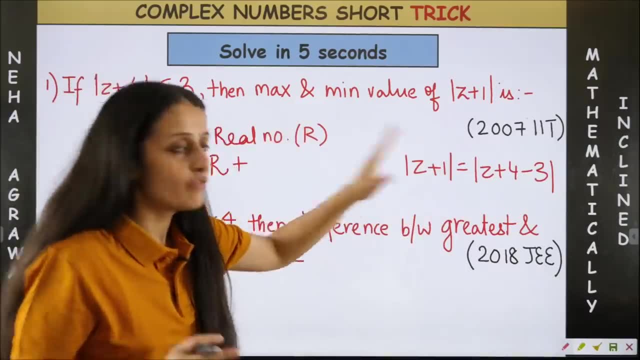 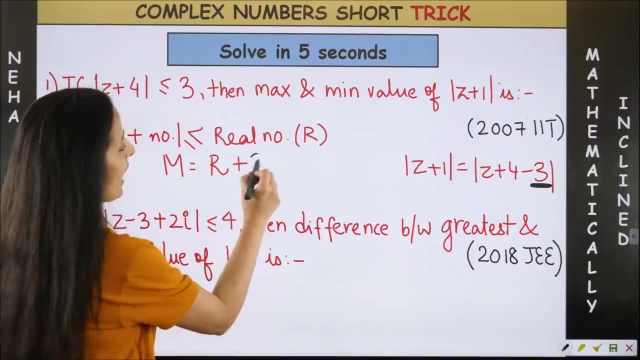 can be expressed in terms of this as z plus 4 minus 3.. Look, the idea is to introduce mod of z plus 4, but at the same time, overall this should stay 1.. Okay, Okay, So modulus of this number, which is just 3.. So r plus 3 is the maximum value and r minus. 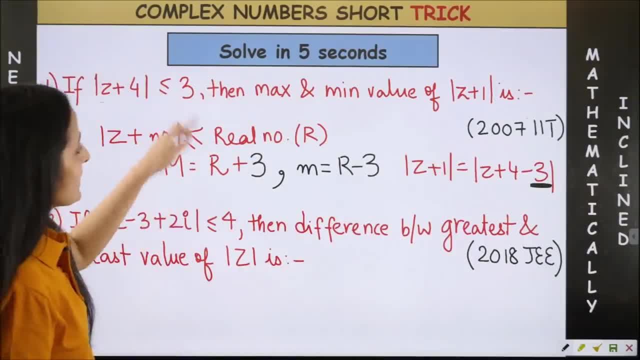 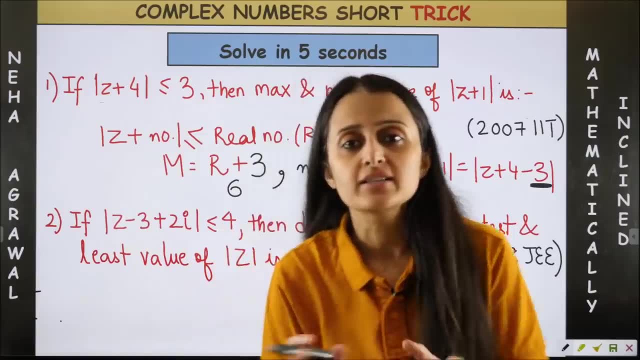 3 will be the minimum value. That's it. So in this case it is 3 plus 3, which is 6, and 3 minus 3, which is a 0. So I know it's based on a very, very simple concept, but trust me, 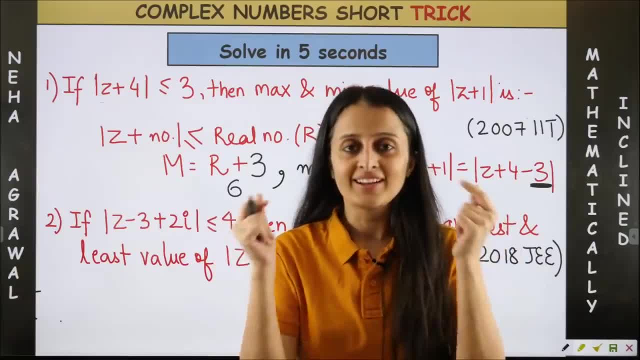 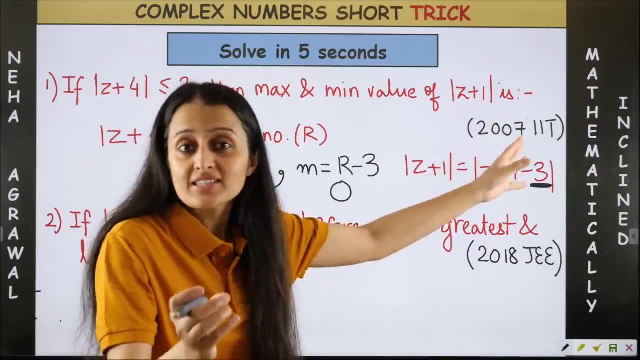 by applying this, you can crack such problems in a jiffy and, as you can already see, the problems that are there are very simple. So what I have taken to begin with are from your 2007 AIEEE and your 2018 online JEE. 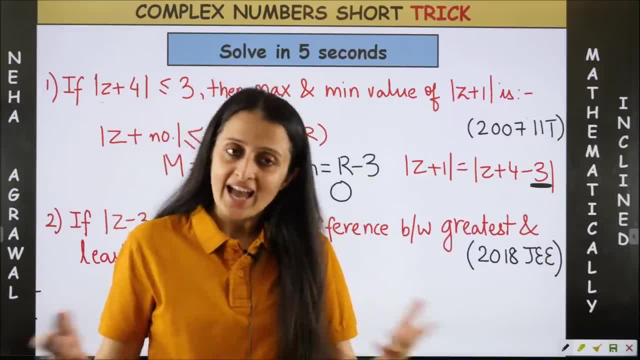 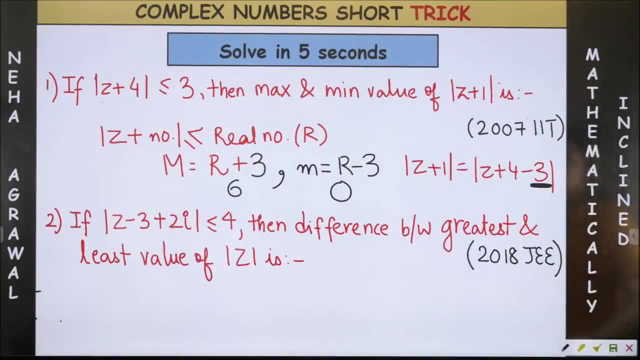 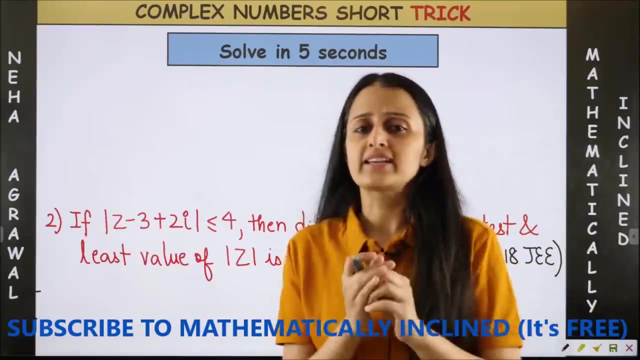 Means these questions have occurred in the past and can be a part of your new JEEE as well. Please make a note. Let's create this magic for the second question Now. in the beginning you may find that it might take you till 10 seconds, but once you understand the whole thing, trust me this. 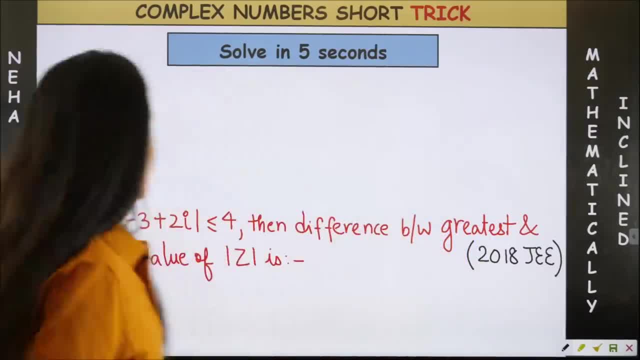 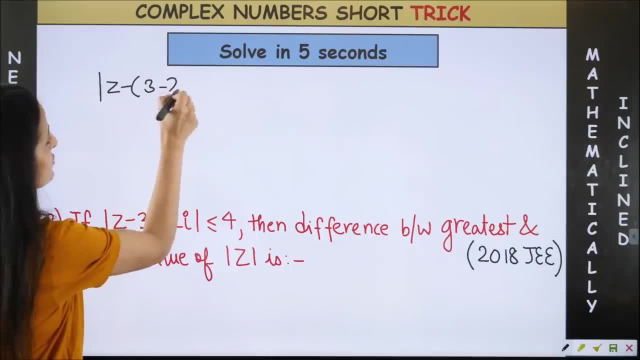 is going to come down to less than 5 seconds as well. So now you are given the same structure, which you can even write it as: z minus 3 minus 2i- right is less than equal to 4.. That means: 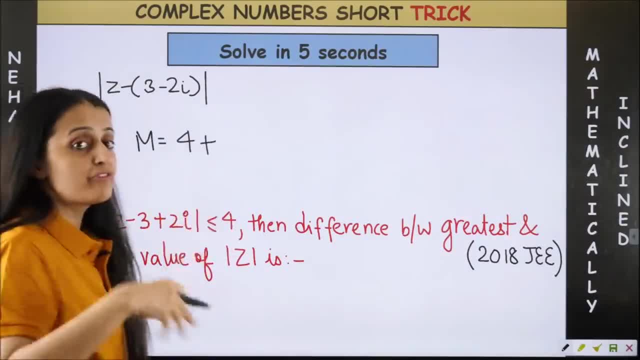 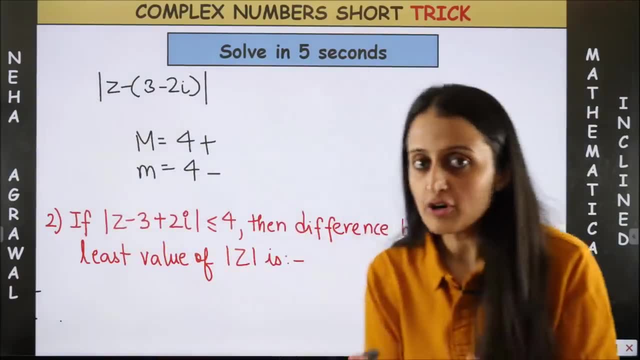 simple si kahani hai boss. My maximum is going to be 4 plus something, and minimum is going to be 4 minus something. Now just realize one thing: Of course you will be given the options in MCQ questions. So if you are given the options, you will be given the options. So if you are given 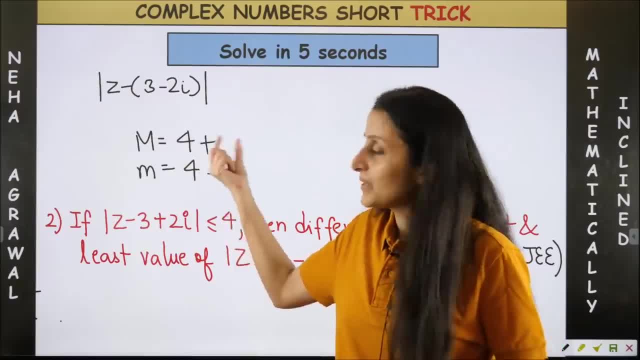 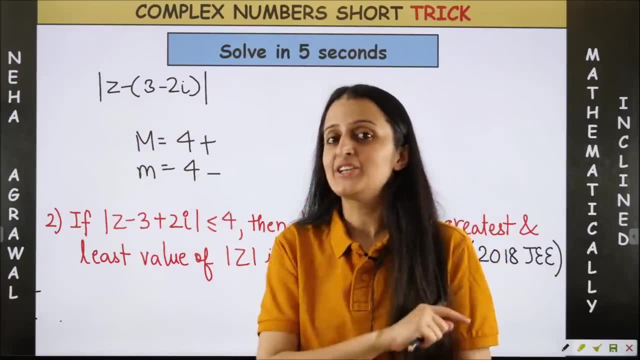 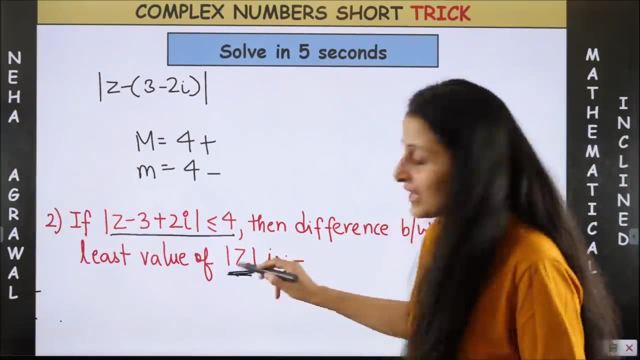 the options. you can chuck out those options if something is giving you lower than 4 for maximum, and likewise whatever for minimum. So you can eliminate options. For now, you know that this is what is given to us and this is where we have to reach. So, in order, 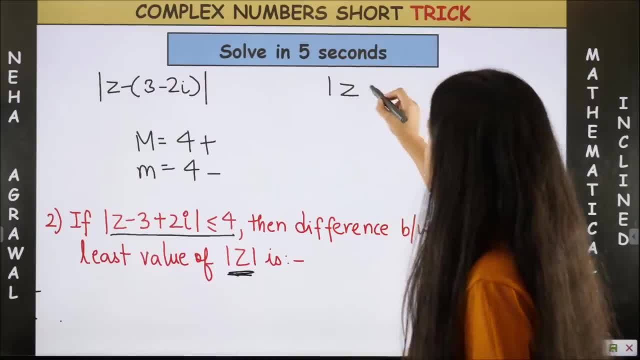 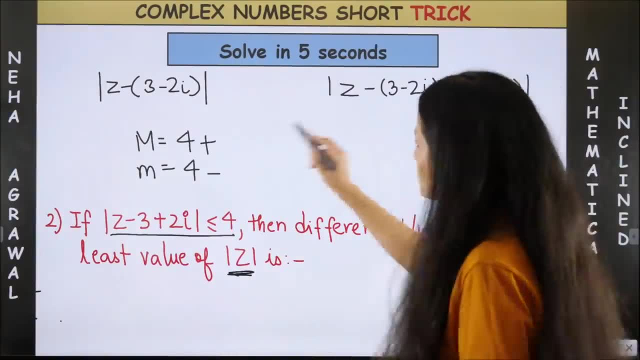 to express your mod z, of course, you can write it as z minus 3 minus 2 iota and to balance it out: plus 3 minus 2 iota, right? So this is what we have to do. So this is what we have to do, So, in order to express: your mod z, of course. you can write it as z minus 3 minus 2 iota, and to balance it out plus 3 minus two iota, and to balance it out plus 3 minus two iota. and to balance it out plus 3 minus two iota and to balance it out. So this is 4, and now I only have to focus. 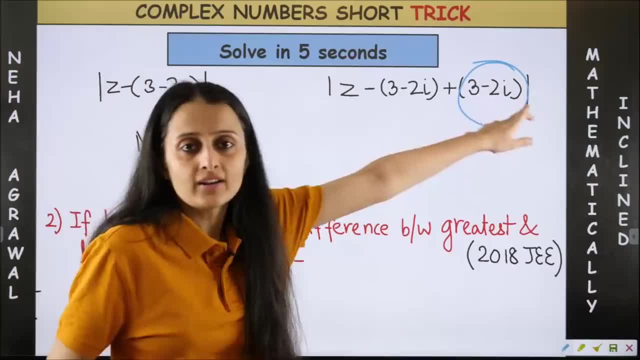 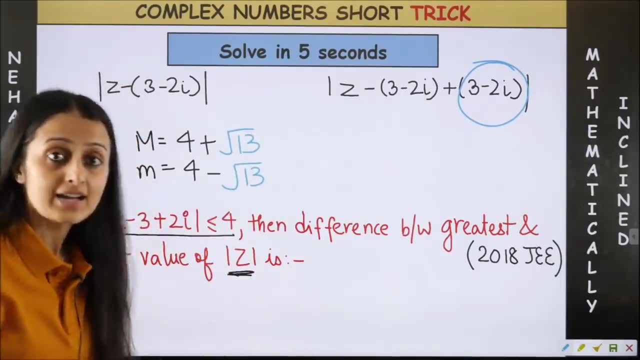 on the modulus for this which you can do mentally: 3 square plus your 2 square, which is root 13.. So 4 plus root 13,, 4 minus root 13 is the answer. But, but, but, baccho, if you have. 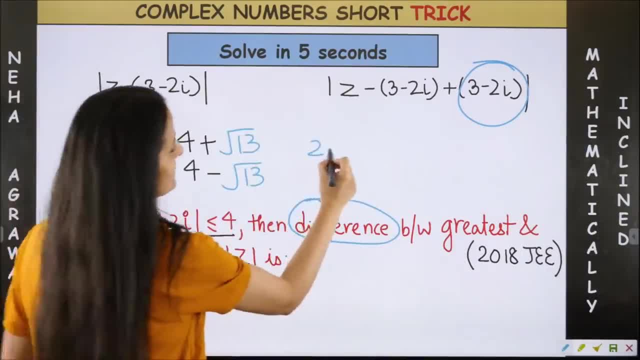 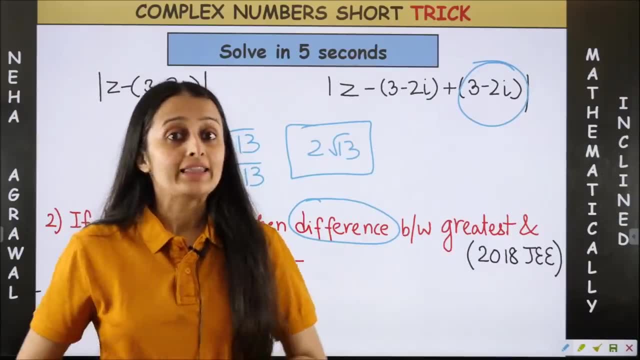 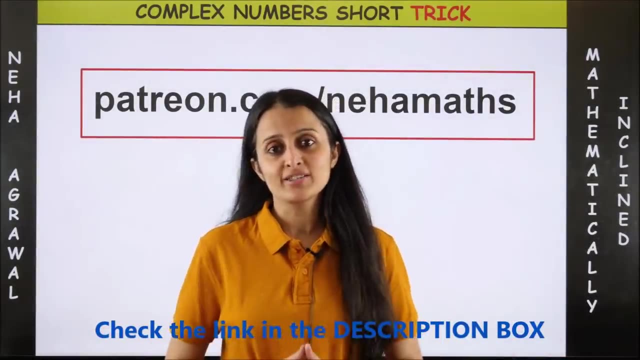 been asked to find a difference. then you clearly can see the difference is going to be 2 root 13.. Bingo, That's how simple it was. Make a note and then we will go ahead. Hey guys, now you can support us on Patreon as well. This link will also be available in the. 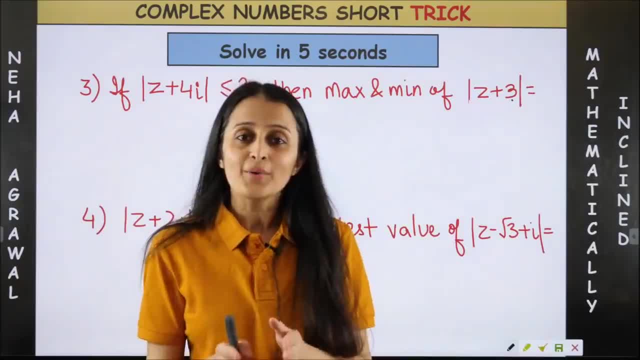 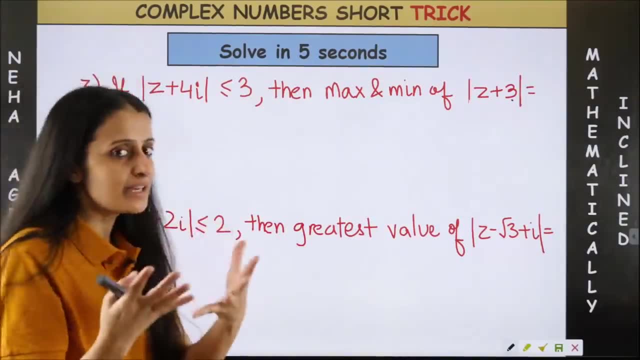 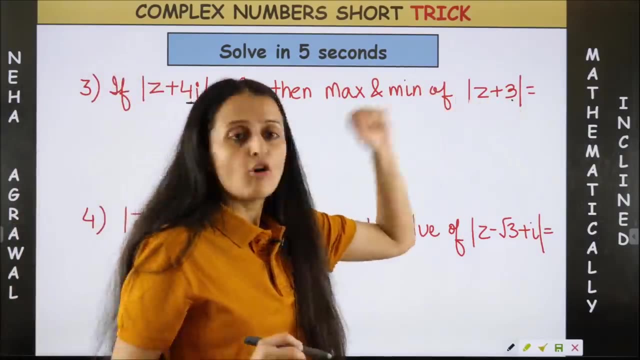 description box below. So check it out. Now let's go further and dissect two more problems. So look at the first one. It is again the similar pattern. Mod of z plus 4 iota is less than equal to 3.. Then maximum and minimum of mod of z plus 3 is. So now just watch it out. You already know. 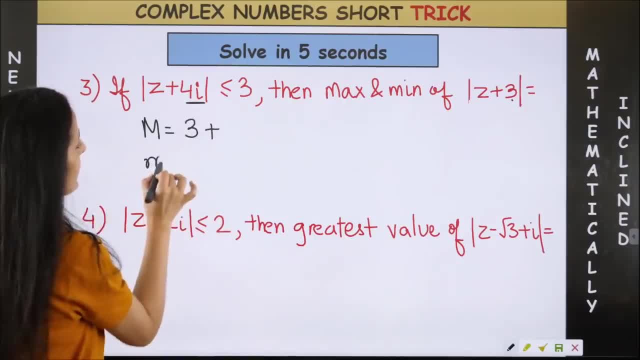 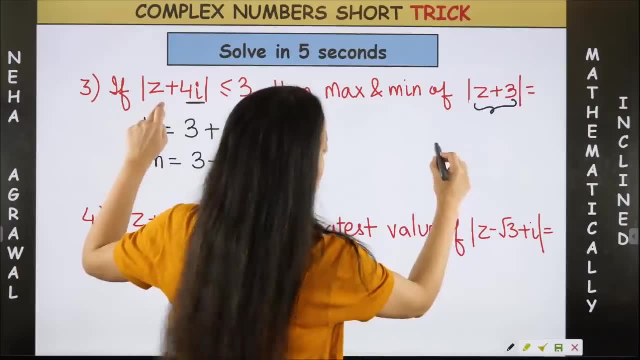 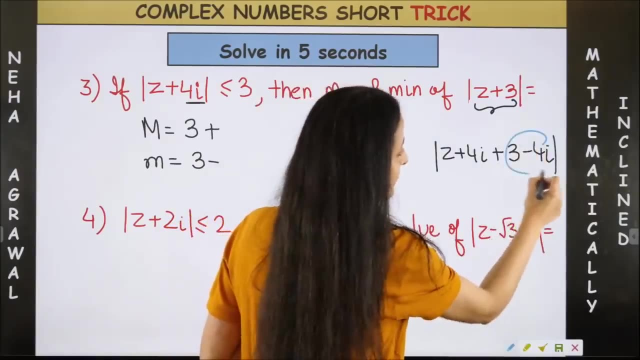 that your final answer is going to be 3 plus something and minimum is going to be 3 minus something Here for z plus 3, now all you need to do is, in order to create this plus 4i, right, and minus 4i. That means, if I take the modulus for this one, do it mentally. you know, 9 plus 16,. 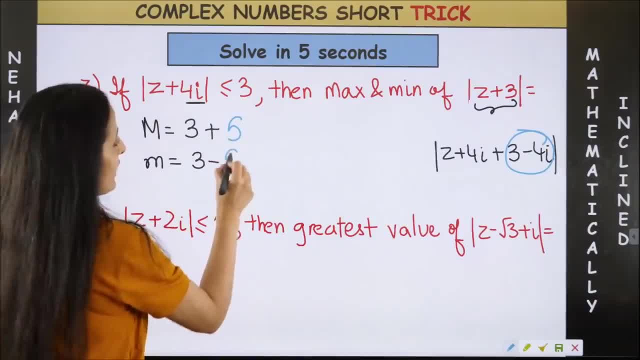 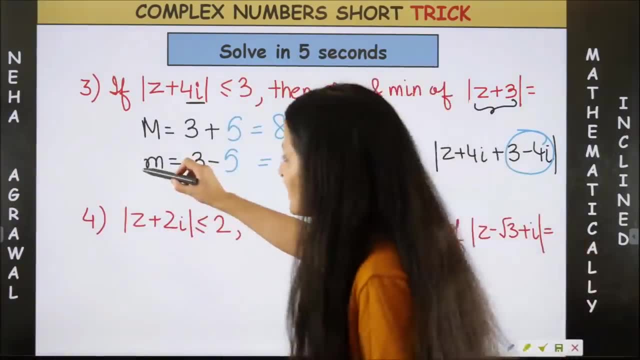 that's 25.. Root of that so gives us 5 and 5. This is 8, this is minus 2.. But come to think of it, we are talking of distances. So that means in case, even if it's negative, you are always. 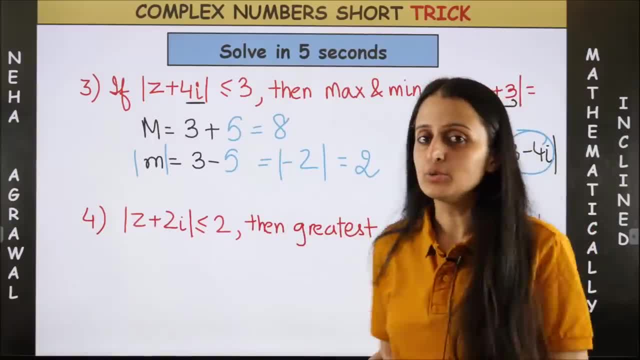 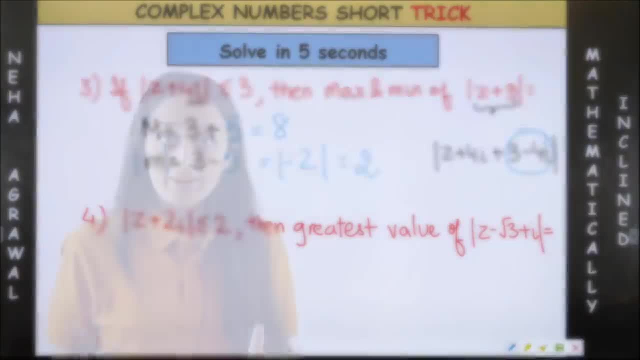 supposed to give the positive answer. So 8 and 2, that's it, The question is dead. One more time, Please make a note Ready for some more action. Alright, here we go. So mod of z plus 2 iota is: 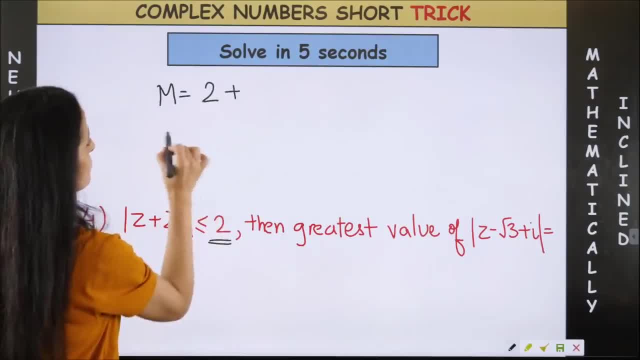 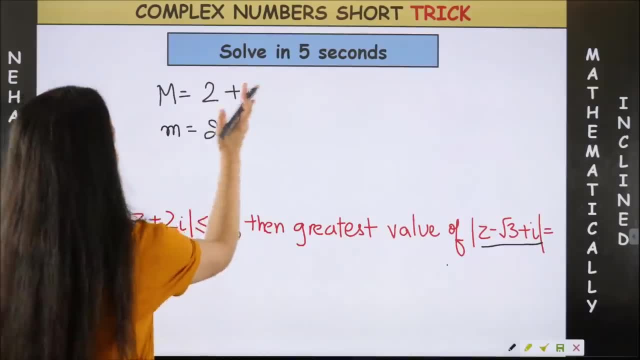 less than equal to 2.. Yani ke, this is going to be 2 plus something and this is going to be 2 minus something. Simple, Now, greatest value. Okay, So we have only been asked greatest value, right? So what will I get? 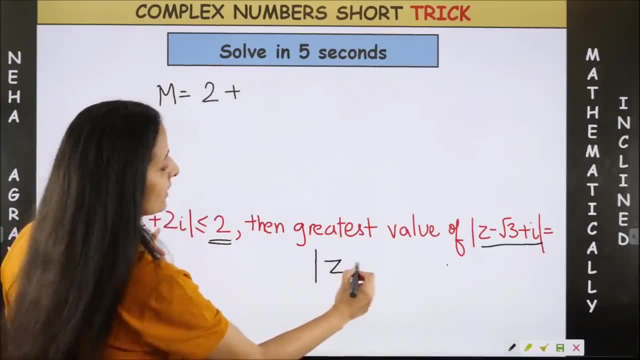 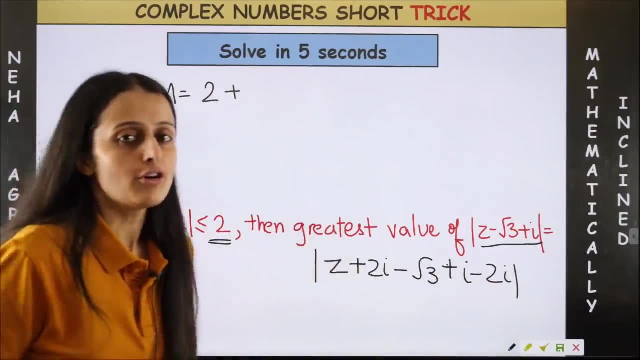 This can be expressed as mod of z plus 2i, and this is minus root 3 plus i minus 2i. See, I am trying to show all the steps, but of course you can do all these things mentally as well. 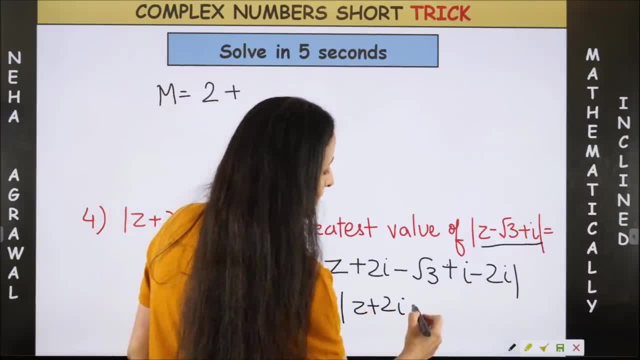 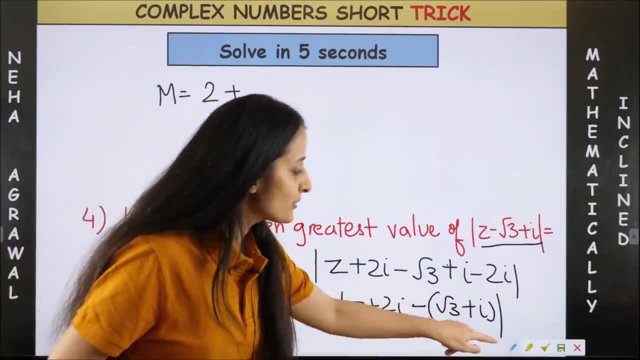 So z plus 2i and this one becomes minus root 3 plus iota. I don't have to care about the minus sign. All I need to care about is the modulus For this one, which is going to be 3 plus. 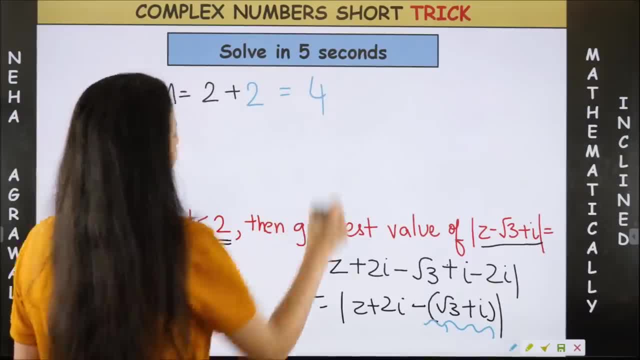 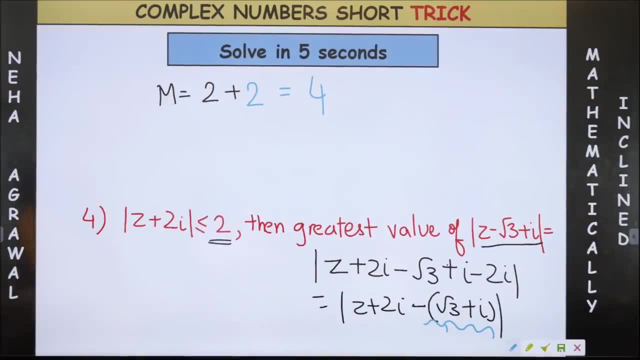 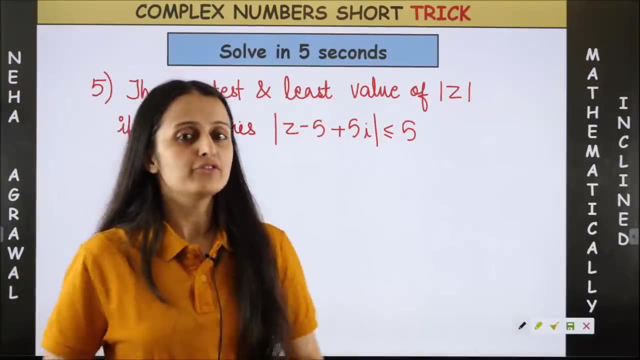 1, 4.. So 2.. So 2 plus 2 is simply a happy 4.. That's it, The job is done. Please make a note: Ye dil manga more To ye do ek, or Let's check out how well versed have you become with this method. 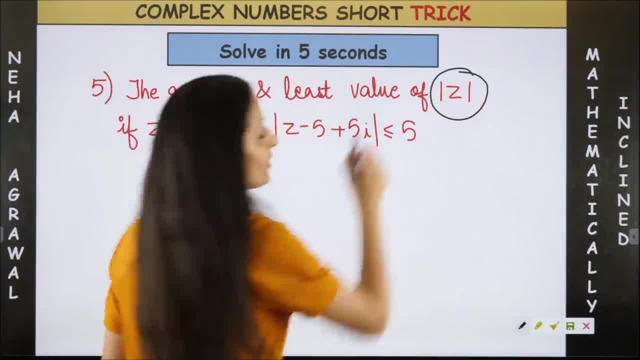 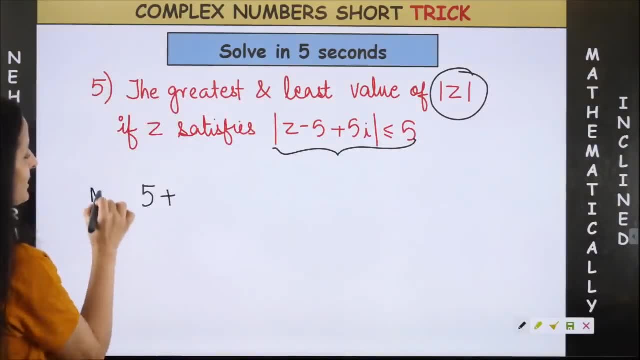 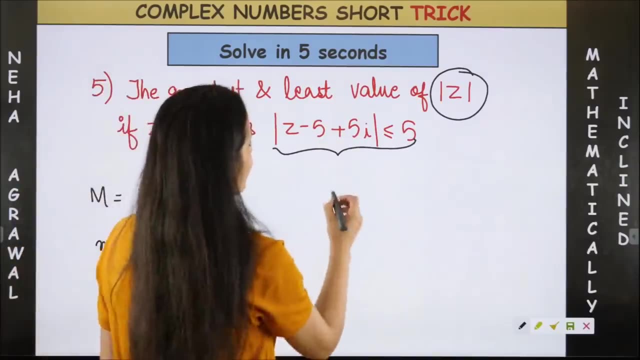 So the greatest and least value for mod of z z when z satisfies this one. so pata hai, boss. my answer is going to be 5 plus something, and for minimum, 5 minus something. hai na now, what is this? something, something. so here i. 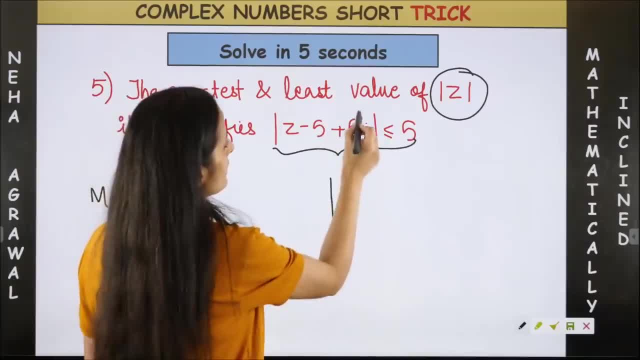 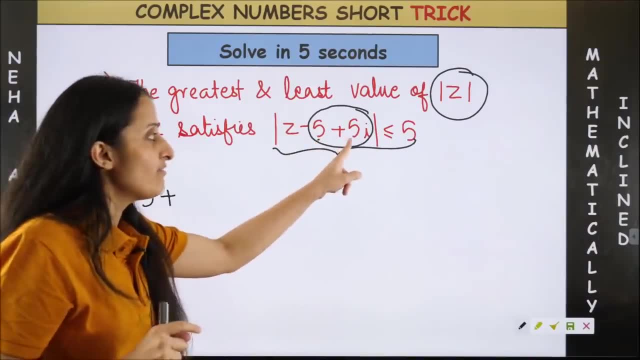 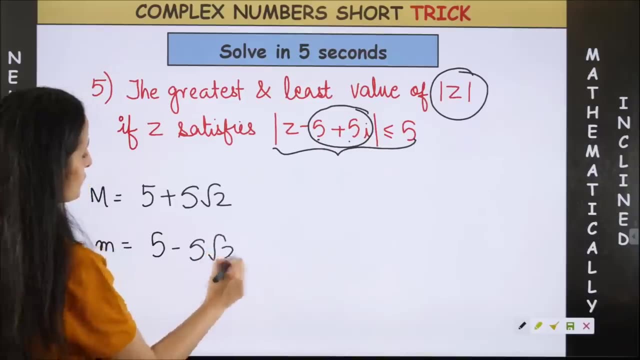 can write. now, this one doesn't have anything, so bingo. that means i just have to find the modulus for this one to mentally karo ya litke. this will be 25 plus 25 makes it 50 root 50, 5 root 2. so 5 plus root 2, 5 minus 5 root 2. just put this absolute value sign here and